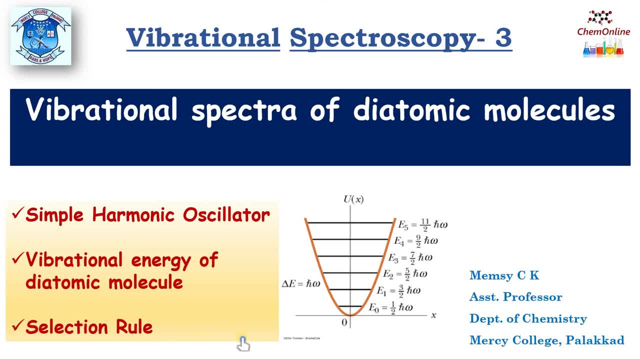 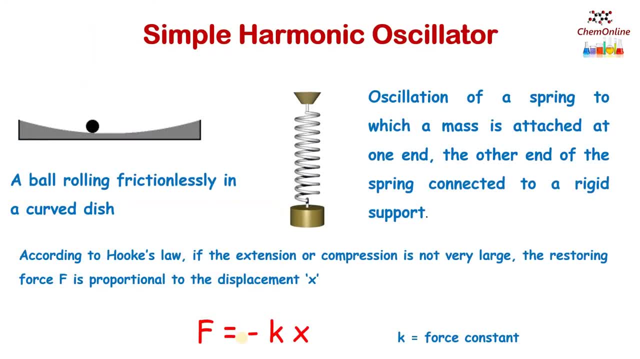 Dear students, in this class we will discuss about the vibrational spectra of diatomic molecules. Before explaining the vibrational spectra of diatomic molecules, first let us see what is meant by a simple harmonic oscillator. Any device that interconnects potential energy and kinetic energy repeatedly is an oscillator. For example, a ball rolling. 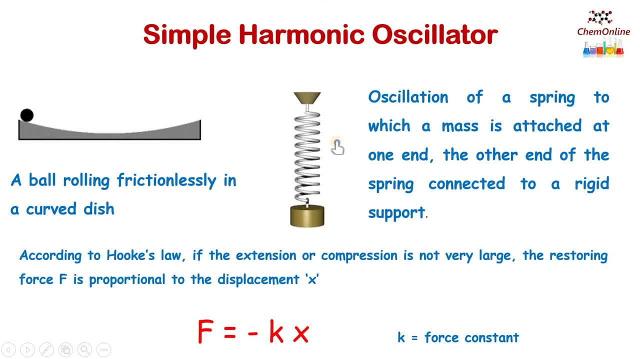 frictionlessly in a curved dish, or the oscillation of a spring to which a mass is attached at one end, the other end of the spring connected to a rigid support. These two are examples of systems which exhibit harmonic oscillation. The motion of a simple pendulum is another example. 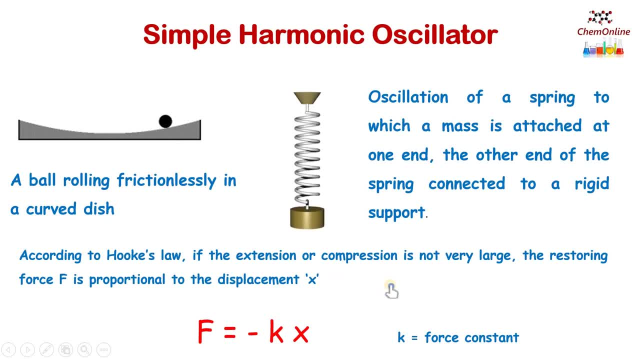 In simple, harmonic motion. when a particle is displaced from its equilibrium position, a force starts acting on it in the opposite direction in order to restore it towards equilibrium position. This model was proposed by Hooke, So according to Hooke's law, 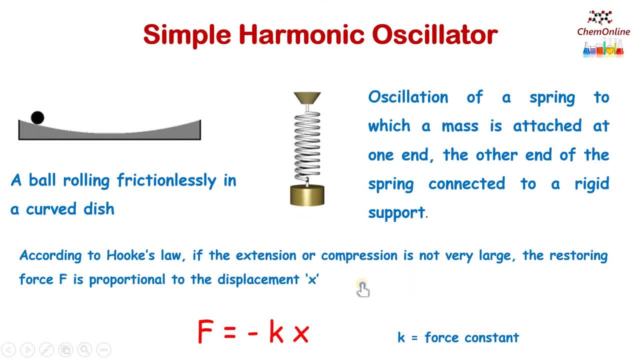 if the extension or compression is not very large, then the restoring force F is proportional to the displacement x. That is, F equals minus k into x. where k is a constant known as force constant, The negative sign indicates that the force is in the opposite direction. So systems which exhibit simple 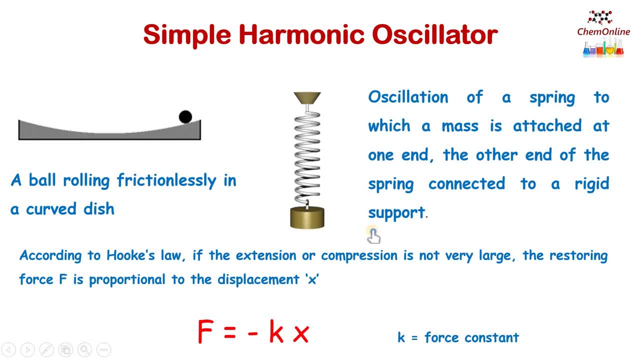 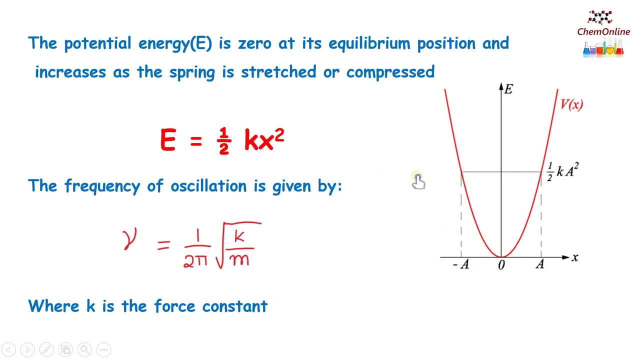 harmonic motion and which obeys Hooke's law are called simple harmonic oscillators. In a simple harmonic oscillator the potential energy is zero at its equilibrium position position and increases as the spring is stretched or compressed, and that is given in this graph, which is a parabola. The potential energy is expressed as: E equals half kx square and the 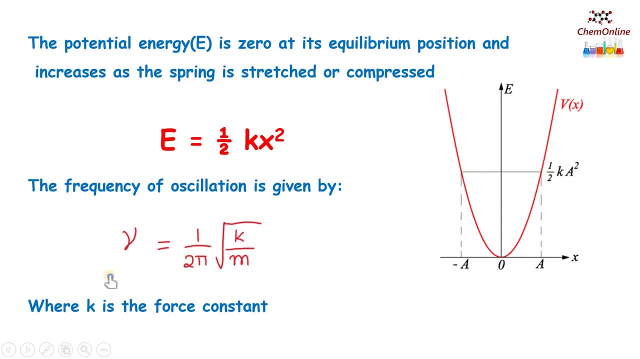 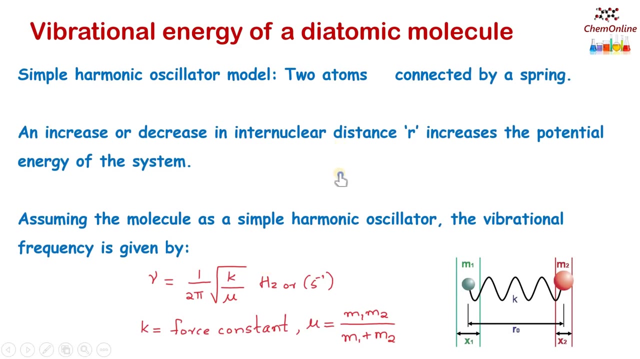 frequency of such a simple harmonic oscillation is given by nu equals 1 by 2 pi, root of k by m, where k is the force constant and m is the mass. Now let's discuss about the vibrational spectra of a diatomic molecule. To explain the spectra, a diatomic molecule is viewed as a simple 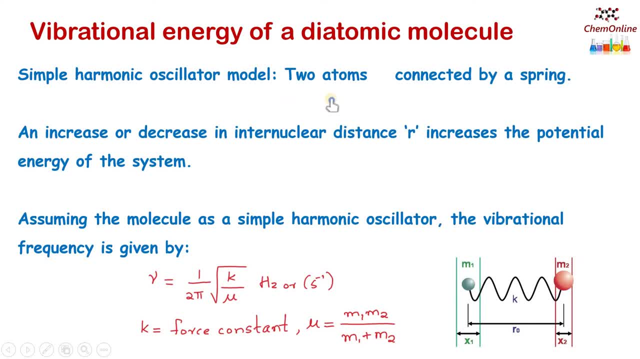 harmonic oscillator. That is, the two atoms are connected by a spring, That is, the bond between the two atoms is like a spring which can be stretched or compressed. So consider a diatomic molecule with atoms of masses, m1 and m2, joined by a bond which is a spring. 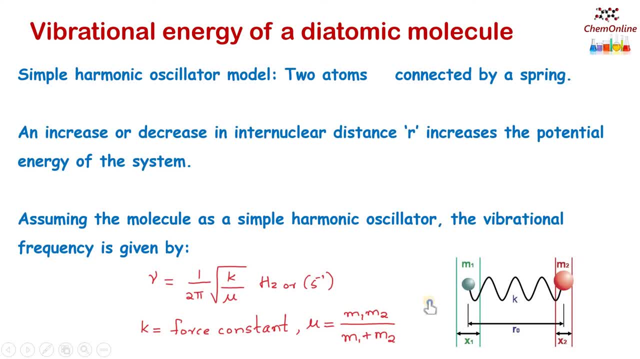 which can vibrate back and forth. Here we are assuming that one atom is fixed and the other is moving away from or towards it. R0 is the equilibrium internuclear distance or the bond length, An increase or decrease in the internuclear distance or? 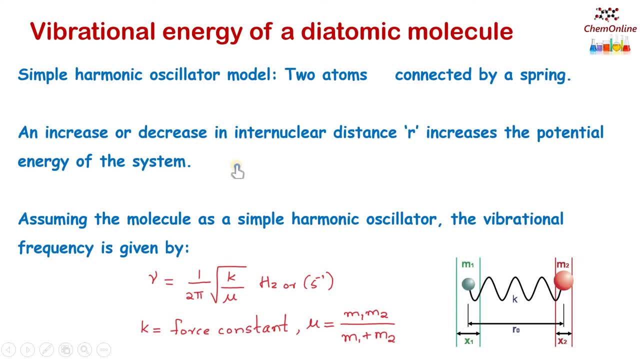 bond length. R increases the potential energy of the system, Assuming the molecule as a simple harmonic oscillator. the vibrational frequency is given by: nu equals 1 by 2 pi. root of k by mu. k is the force constant and mu is called the reduced mass, which is equal to m1, m2 by m1 plus. 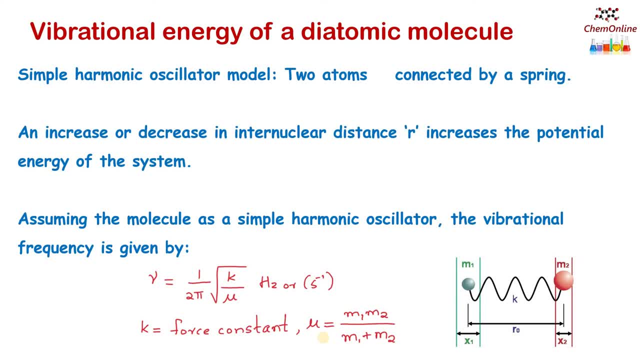 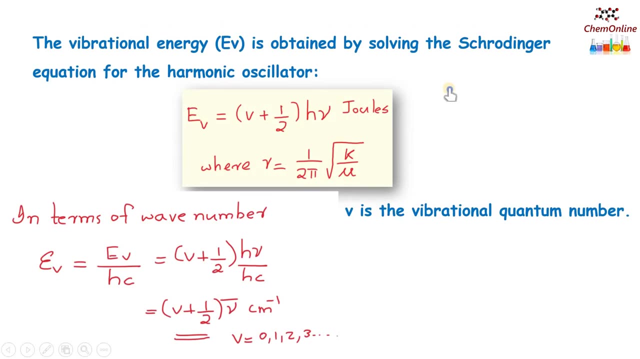 m2.. In the case of simple harmonic motion, the frequency was given as 1 by 2 pi, root of k by mu, where mu is the mass. Here, instead of a single mass, m, we are using the reduced mass. mu equals m1, m2 by m1 plus m2.. Now we have to find out the vibrational energy, and that is obtained by: 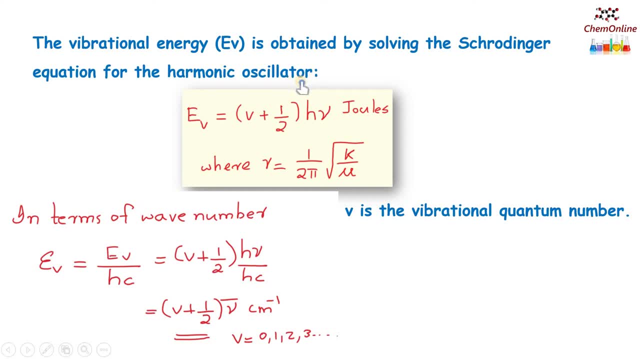 solving the Schrodinger wave equation for harmonic oscillator and the vibrational energy is given by: e equals v plus half into h nu joules, where nu equals 1 by 2 pi root of k, k by mu, and v is called the vibrational quantum number and its values range from 0,, 1,, 2, 3, etc. 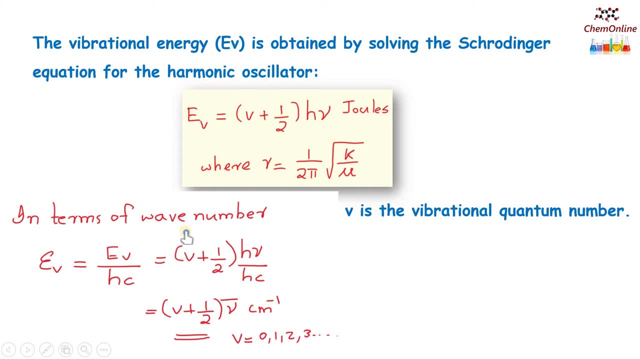 We can also express the energy in terms of wave number. So in terms of wave number, we can write epsilon: v equals e by hc, which is equal to v plus half, h. nu by hc, that is equal to v plus half, into nu bar, where nu bar is the wave number. So v plus half nu bar, centimeter inverse. 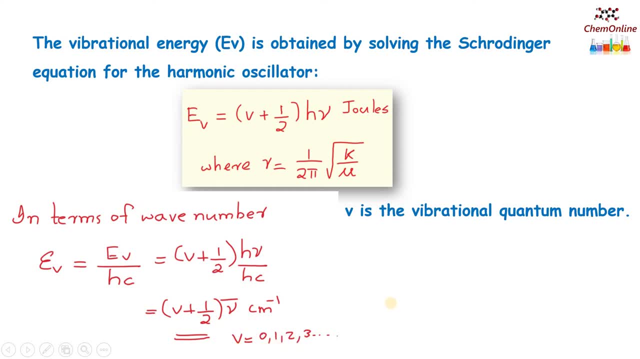 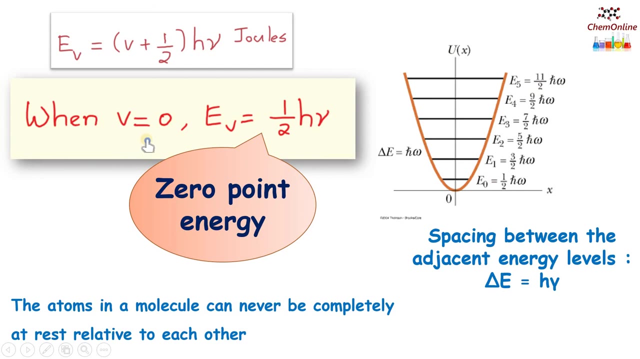 v equals 0,, 1,, 2,, 3, etc. So this is the vibrational energy of a diatomic molecule and the vibrational energy is quantized In the equation for vibrational energy. if we put v equals 0, then we get e equals half h nu. 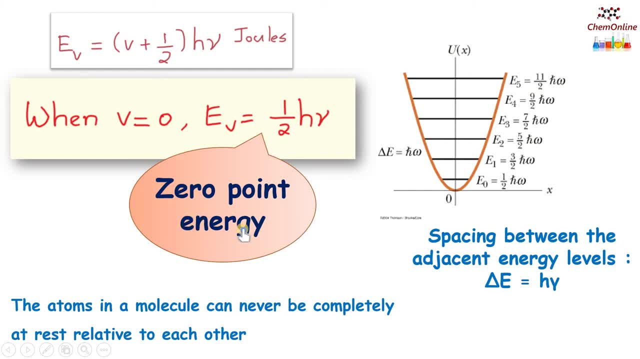 This energy becomes physicalß is called the zero point energy. That is, even in its lowest vibrational level, that is, at v equals zero. a molecule possess some vibrational energy which is equal to half h nu, and that is called the zero point energy. That means no molecule can ever have zero vibrational energy. or we can also: 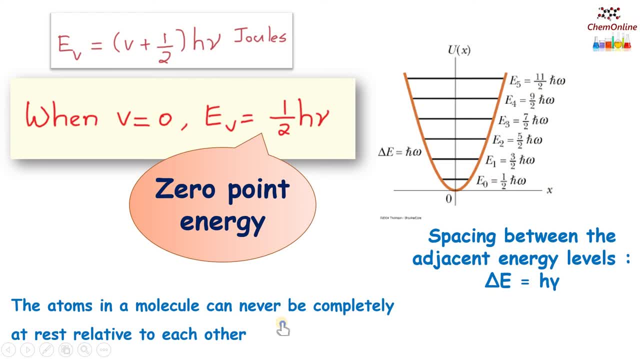 say that the atoms in a molecule can never be completely at rest relative to each other. So even at zero kelvin though, there is no translational or rotational motions, but vibrational motions will continue. If you put v equals 1, the energy will be 3 by 2 h nu. 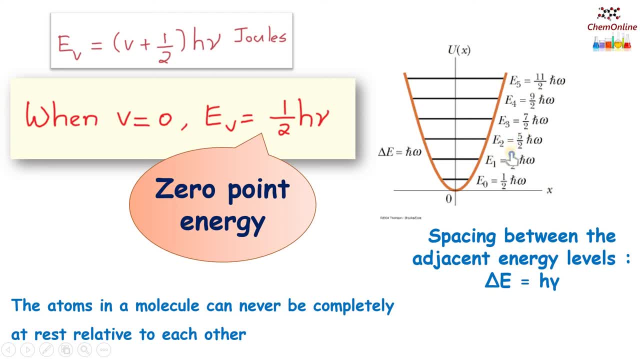 For v equals 2, 5 by 2, v equals 3, 7 by 2.. That means the vibrational energy levels for a harmonic oscillator are all 0. Equally spaced and spacing between the adjacent energy levels will be equal to h, nu, Delta, e. 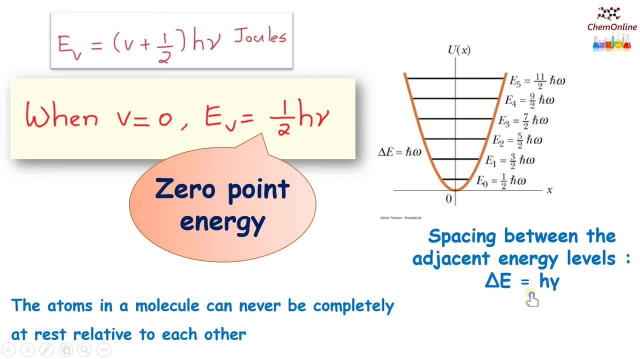 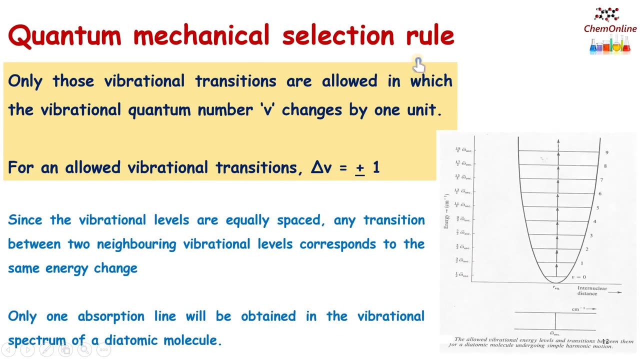 equals. say, for instance, e1 minus e0, that will be h? nu, or e2 minus e1 will be h nu. So the spacing between the energy levels is h? nu and all the energy level, vibrational energy levels, are equally spaced. So from this we can derive a selection rule known as the quantum mechanical. 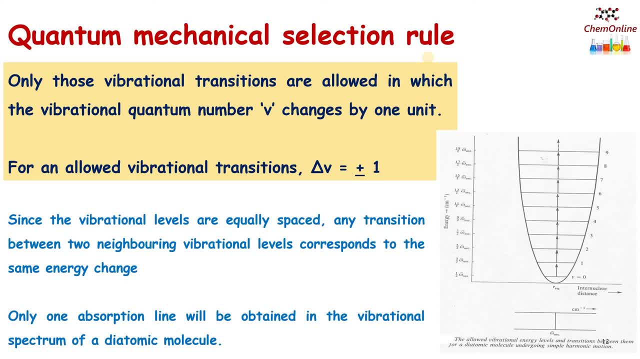 selection rule. We have already seen that the most essential condition for a molecule to show vibrational spectra is that the vibrations must cause a change in the dipole moment. Now this is followed by a quantum mechanical selection rule which states that only those vibrational transitions are allowed. 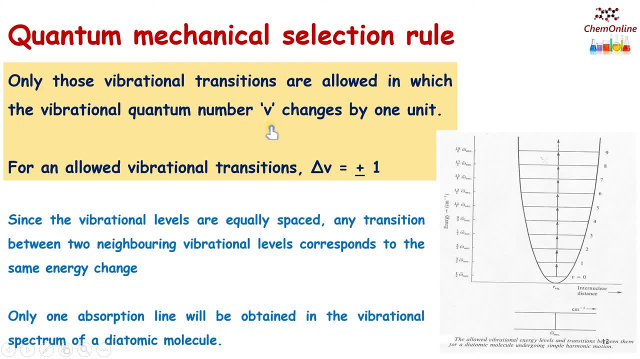 in which the vibrational quantum number v changes by one unit, That is, for an allowed vibrational transitions. Delta v equals plus or minus one. Delta v is the change in the vibrational quantum number. That should be equal to plus or minus one. This is the quantum mechanical selection rule for vibrational